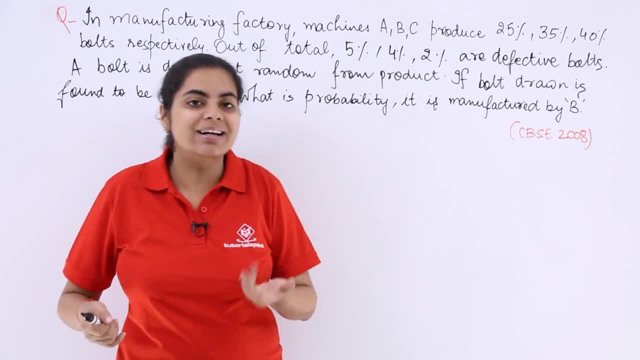 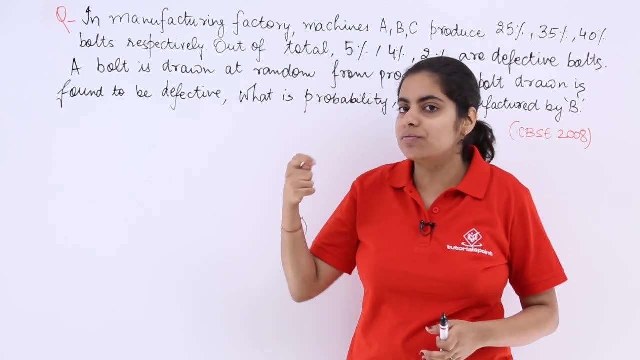 the defective out of the total. A bolt is drawn now at a random from the product. If the bolt drawn is found to be defective, you took out a bolt. If it is found to be defective, what is the probability it is defective? If it is found to be defective, what is the probability it is? 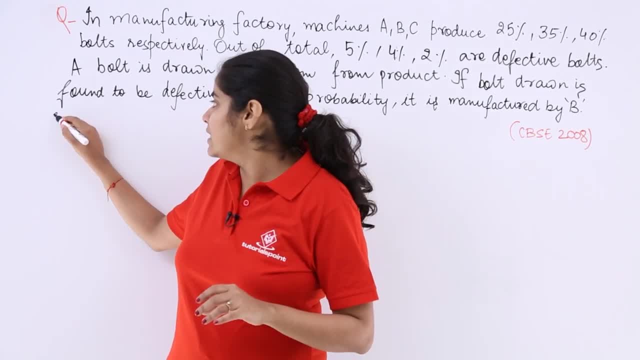 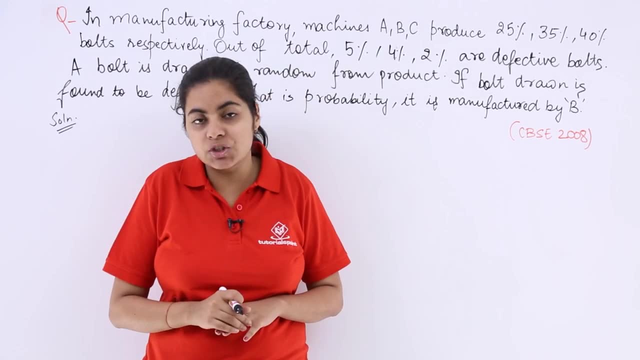 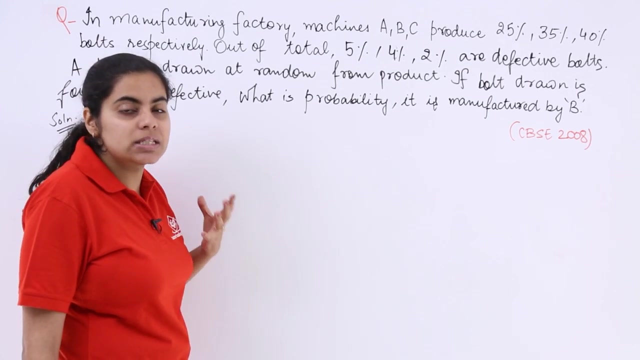 manufactured by the machine B. So let's write solution in step by step. Let's see how to do it. This question is based on Bayes theorem. You see that the definition can be followed, and now let's see how to do it. I know that machines A, B, C are there who are producing certain products. Let I 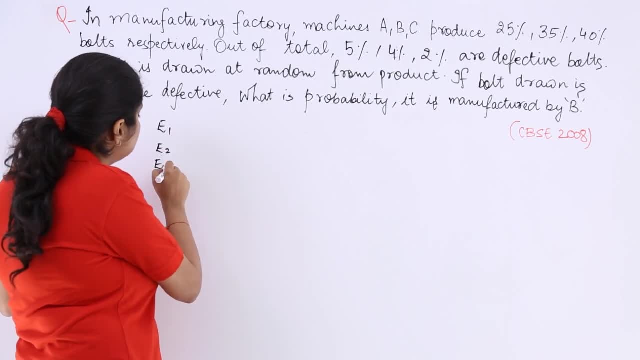 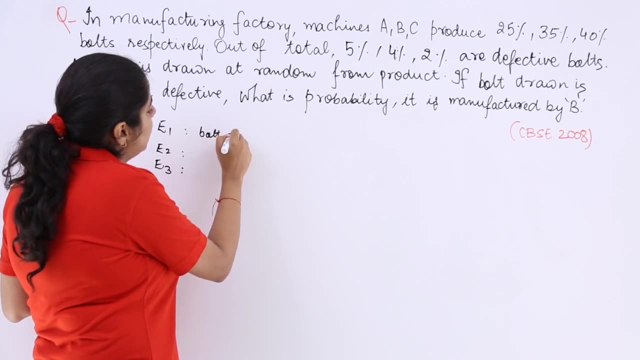 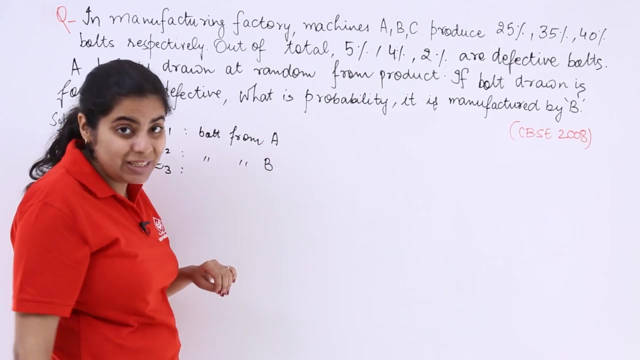 name E1,, E2 and E3 as different events that I am going to take into consideration. E1 says the bolt manufacturing factory is manufactured by the machine B, So let's write solution in step by step. If the bolt manufactured from machine A, E2 says bolt manufactured from machine B, and this: 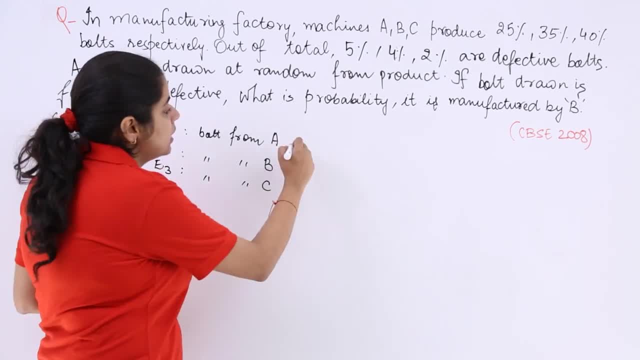 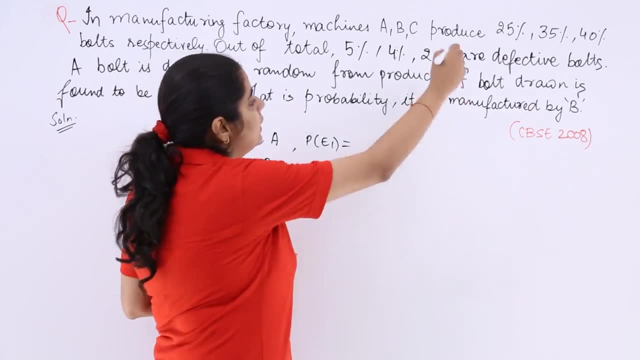 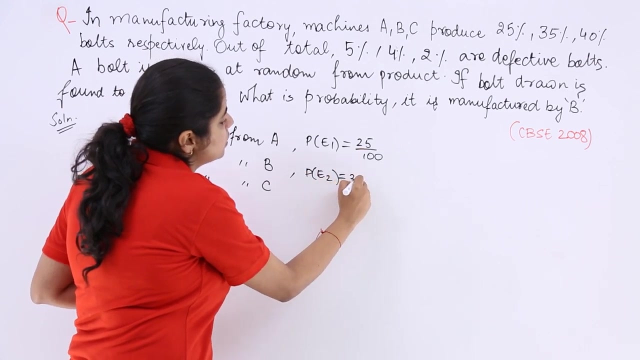 says E3 is bolt manufactured from machine C. Now what is probability of E1? that you are going to manufacture the product from the machine A, and the probability is 25 over 100.. Now what about the probability of E2? Probability of E2 is given to you as 35 over 100.. What about the? 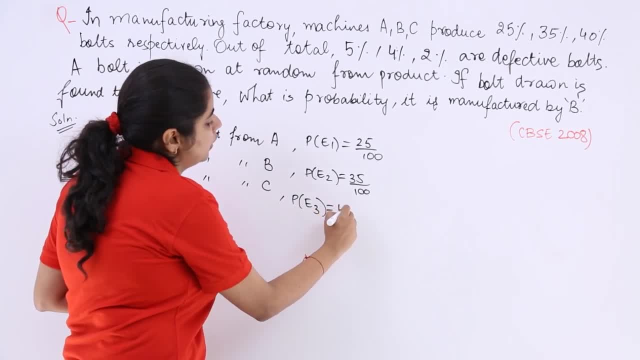 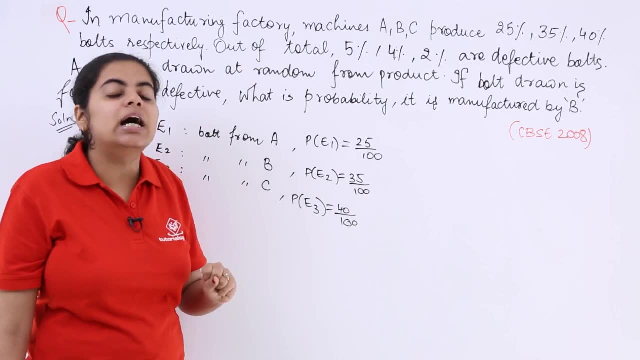 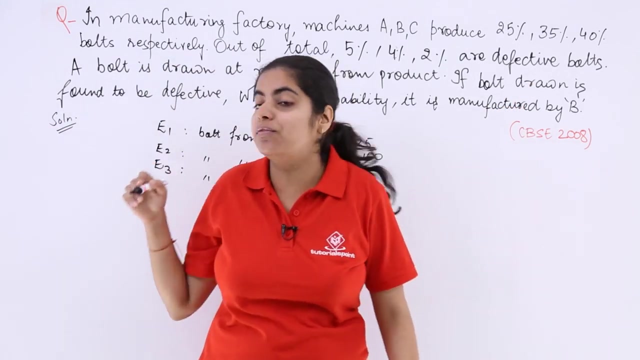 last but not the least, probability P is equal to 40 over 100, so this is done. Now, this is P, P, P. Now we are going to consider, we have to see that if the bolt drawn is defective, so defective bolt probability is also given, so probability of defective. 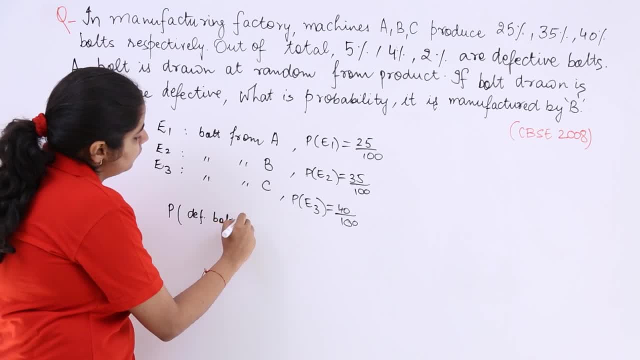 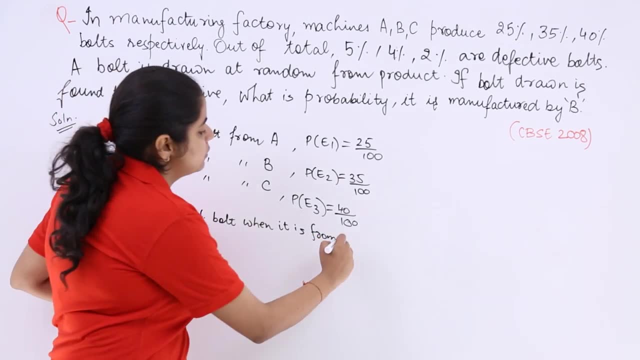 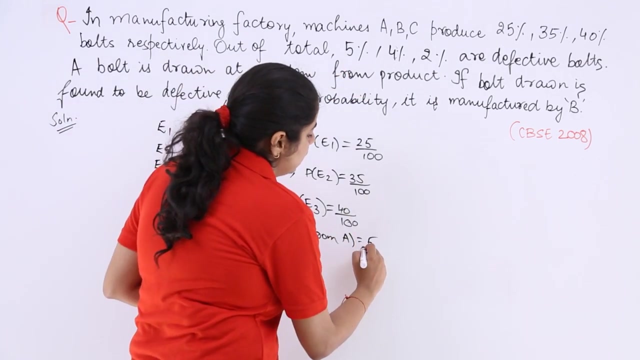 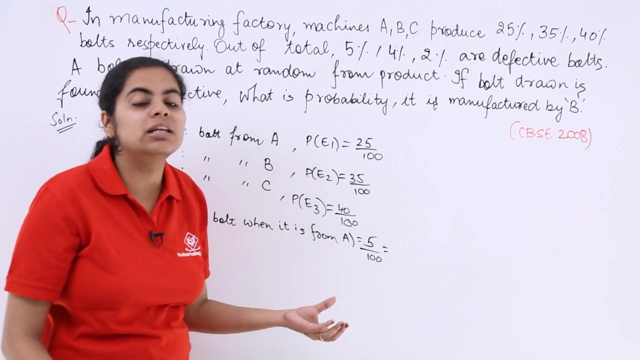 bolt with respect to or when it is from, when it is from machine A. so probability of defective bolt when it is from machine A is 5%, which is 5 over 100. sorry, so this should be 5 over 100, so this is what in mathematical terms. so 5 over 100 is given to you as the probability. 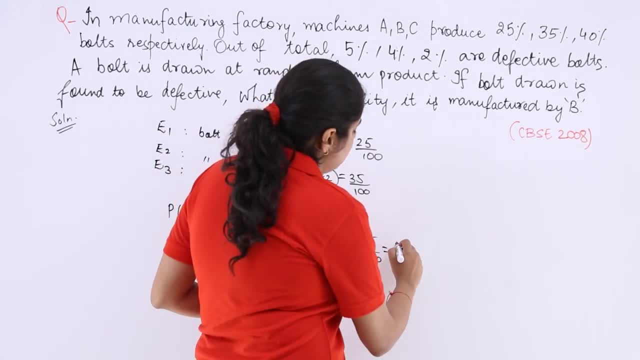 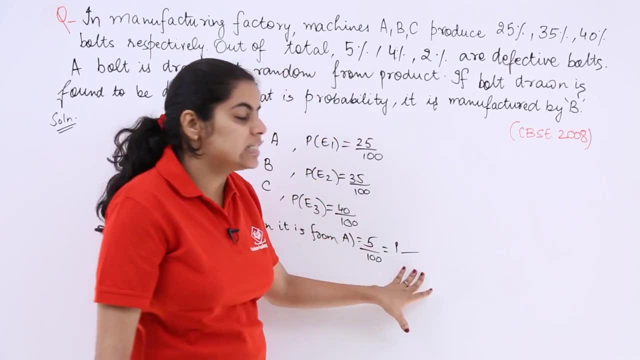 but you see, defective bolt probability is given to you as the probability of defective bolt when it is from A. so it has been known that it is from A and it is defective, right? So from A means you are going to see that since it is defective, let me write: A is the 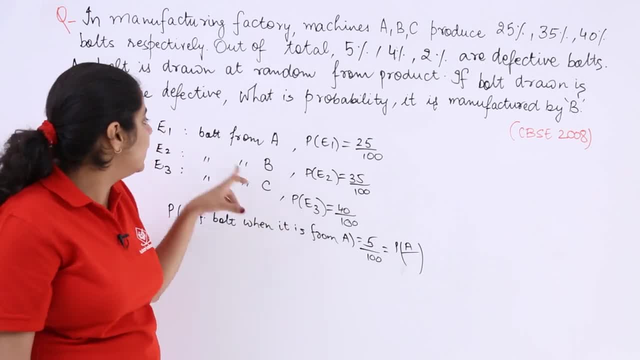 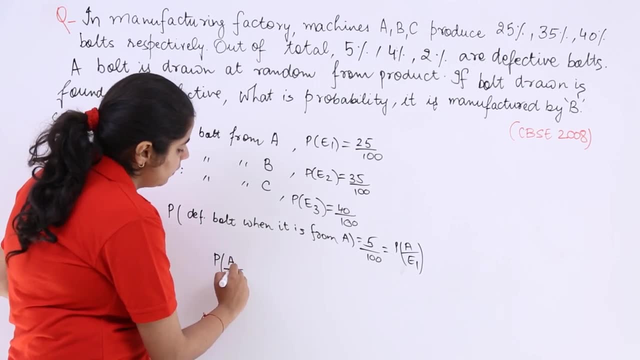 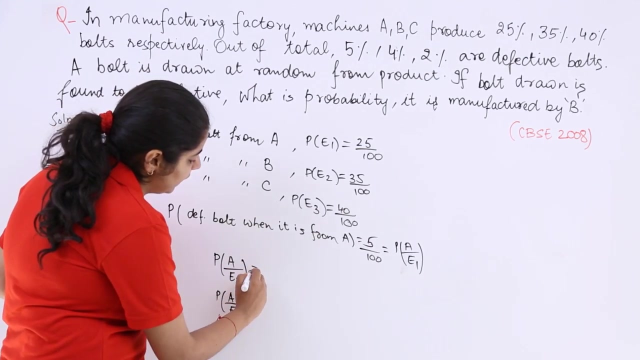 is here which is defective, which says defective, and in the denominator it is to be from machine A, which is E1.. Similarly, if I say it is defective with respect to machine B, similarly it is defective with respect to machine C. So defective means it is denoted by A right. 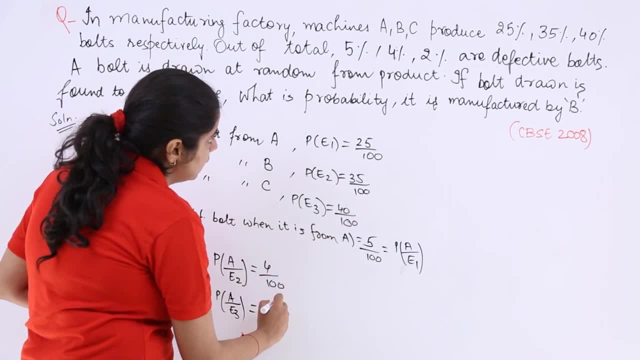 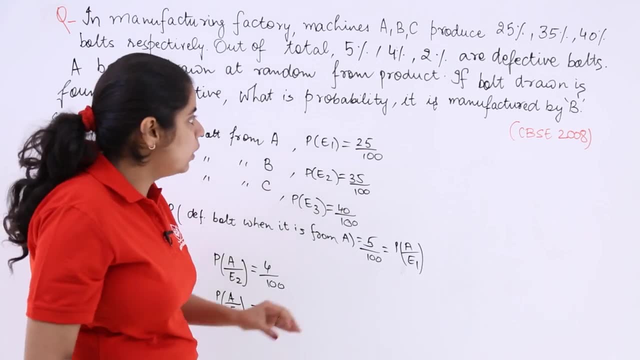 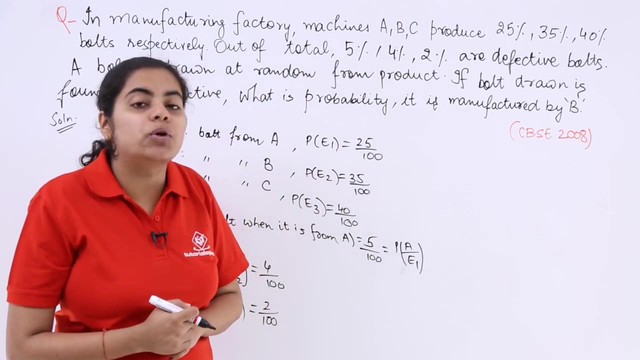 Now what is given to you? 4%, and here it is 2%. so this is the case. Now we have to know that if the bolt is defective, what is the probability? it is manufactured by B. so probability we have to take out that it is manufactured by B. now how to do that? 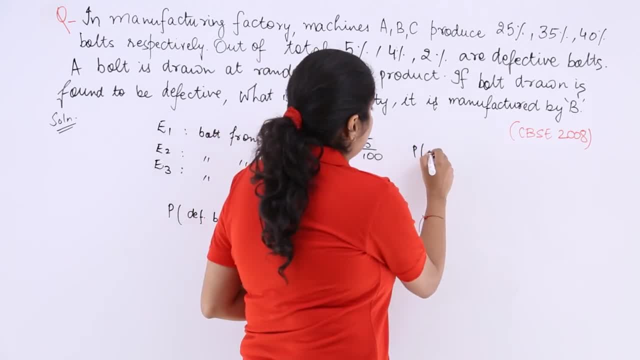 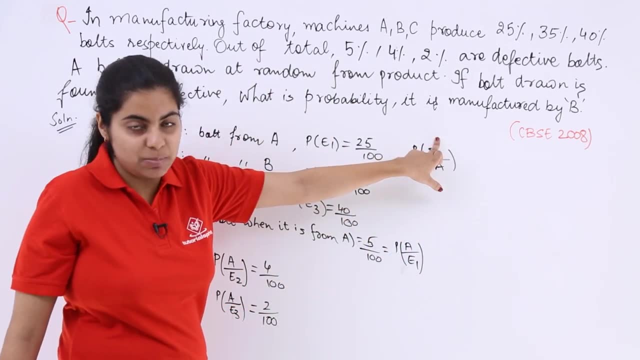 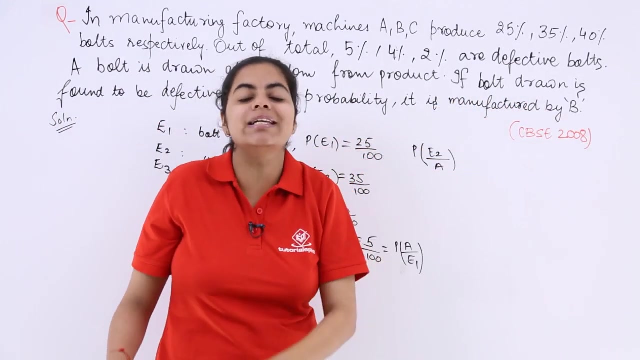 kind of a question. So we have to see: P is a bolt, C is a bolt P of E2 with respect to A, that we have to find out the probability. it is manufactured from B and we know that it has been denoted that the bolt drawn is defective. we have 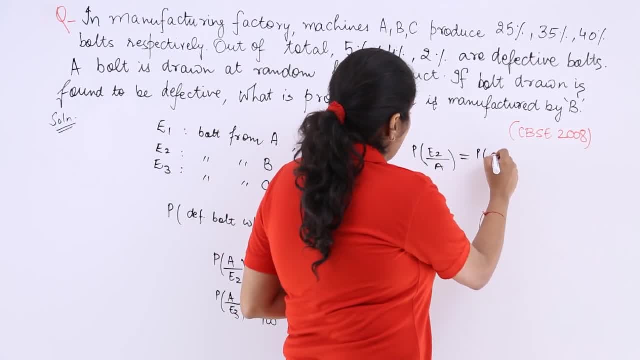 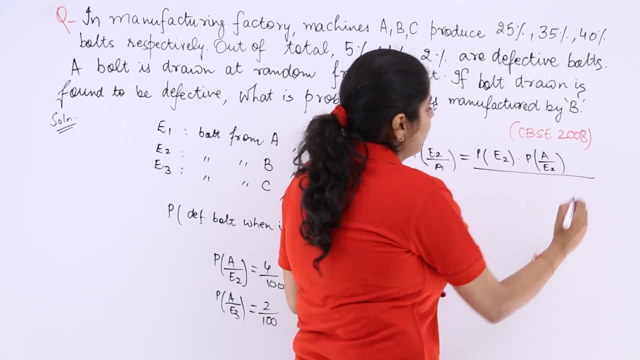 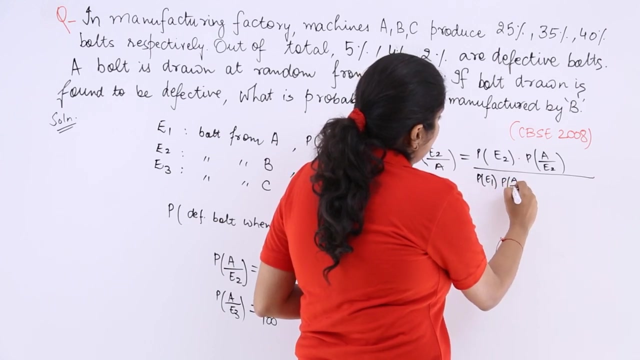 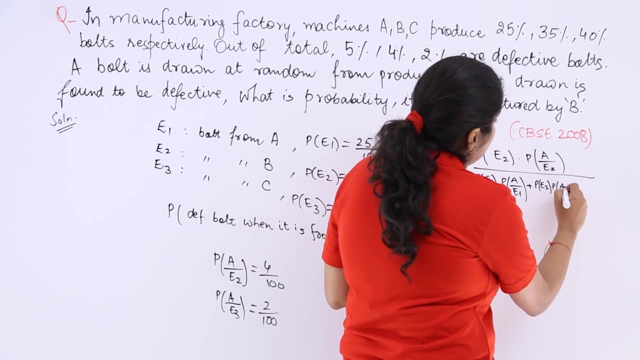 to see Now what is the formula. It should be P of E2, P of A over E2, whole denominator summation in case of Bayes theorem or Bayes theorem. So it will be P of E1, P of A over E1 plus P of E2, P of A over E2 plus P of E3, P of. 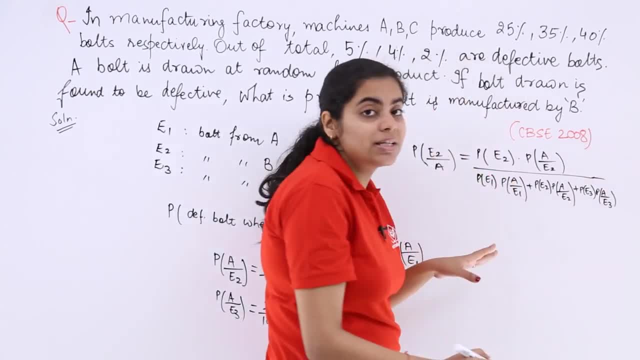 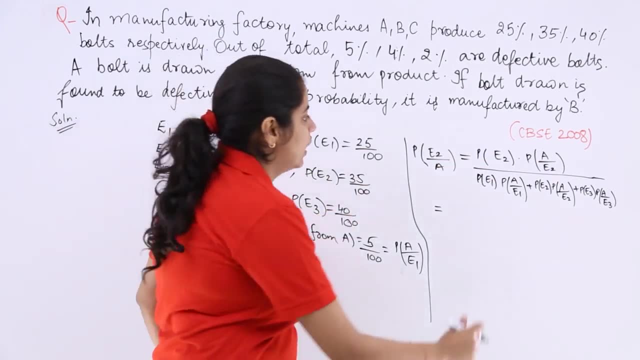 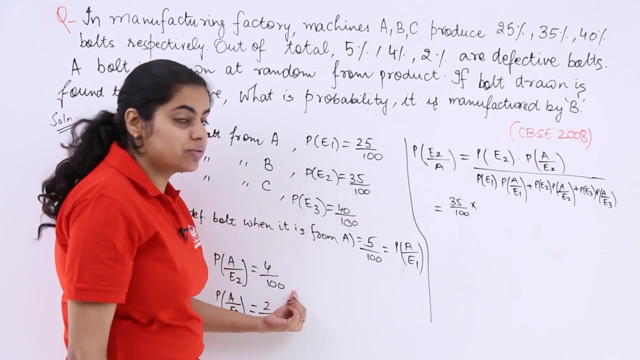 A over E3.. Now what is the answer? Simply, you can put the values and obtain the answer. So P of E2 is what? 35 over 100.. 35 over 100. Multiply by A over E2.. So A over E2 is 4 over 100. 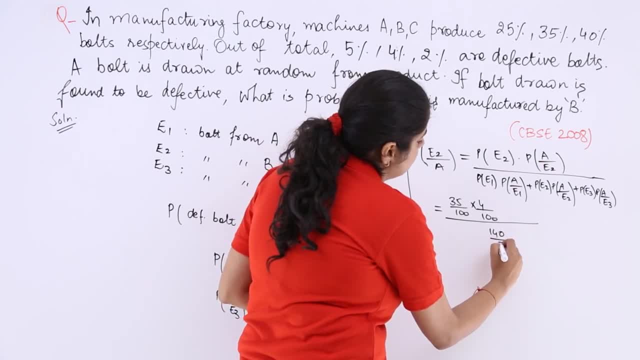 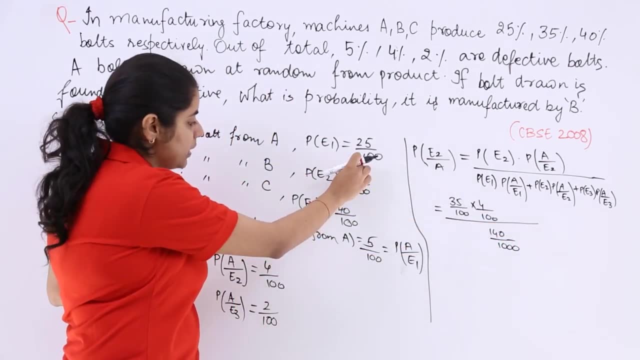 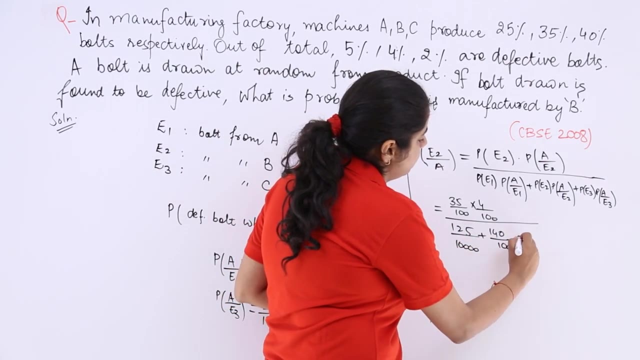 Similarly in the denominator, it will be for this factor. Now, P of E1 into A over E1 means 25, and this multiplied so 125 by 1, with 4 zeros. Last but not the least, E3 and A by E3.